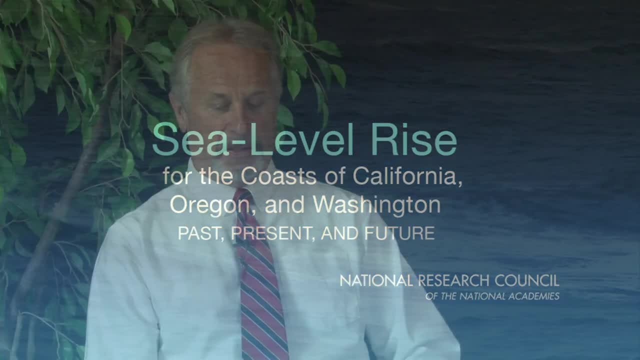 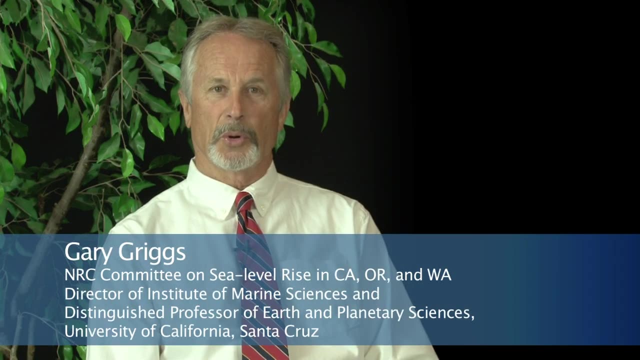 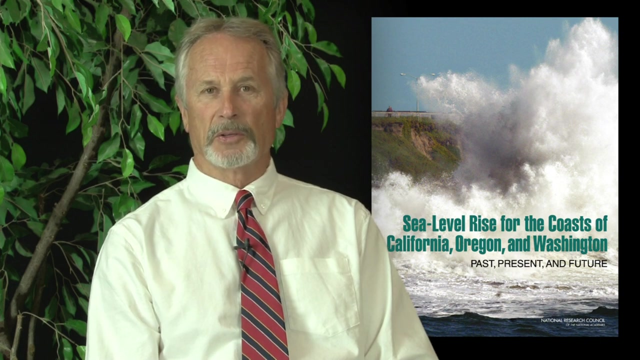 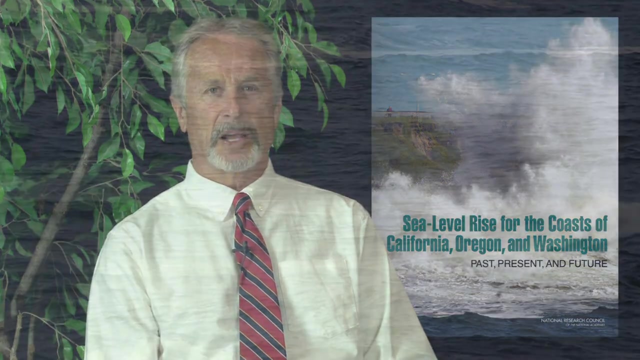 The National Research Council has just completed a new report on sea level rise along the coasts of California, Oregon, Washington, which is intended to provide elected officials, coastal managers and decision makers with an objective and independent analysis upon which they can base future coastal planning. Sea level is rising because the ocean is warming, which 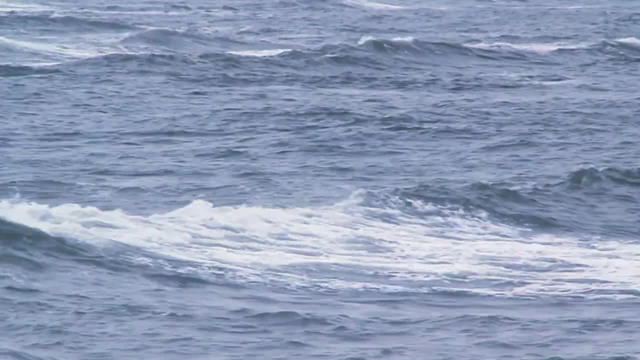 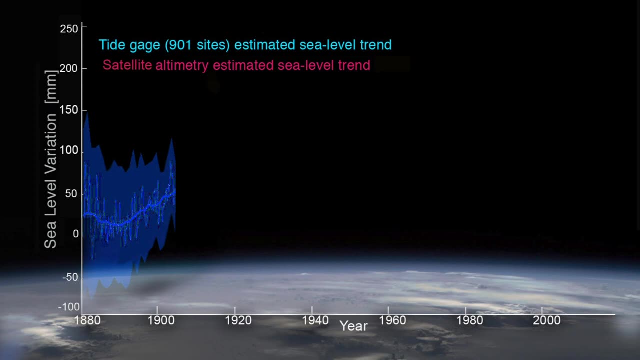 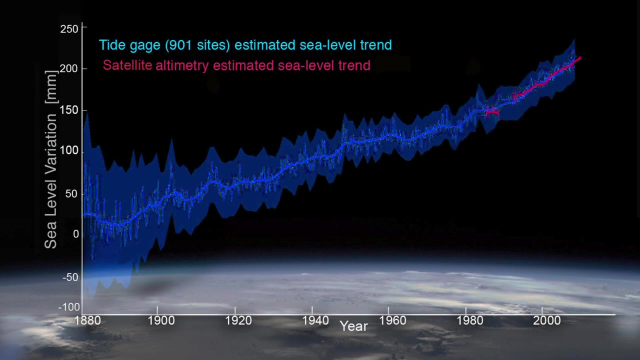 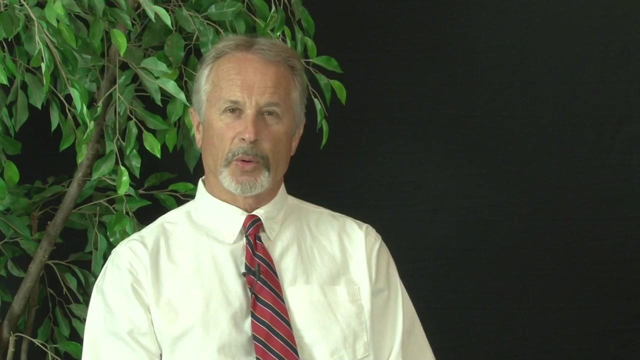 increases ocean volume and also because ice sheets and glaciers are melting. Over the past century, tide gauges indicate that sea level has risen globally about seven inches, But over the last twenty years satellite measurements indicate that number has accelerated to nearly twice as fast as it's been over the last hundred years. So the question is: 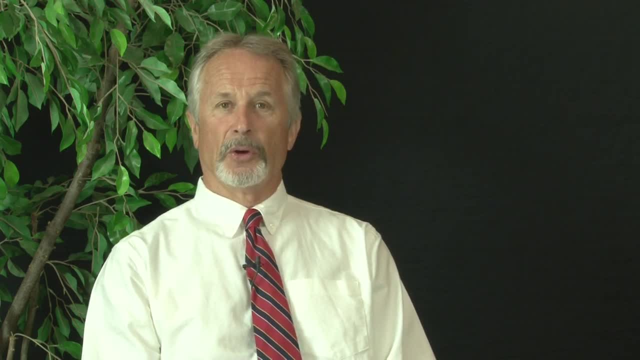 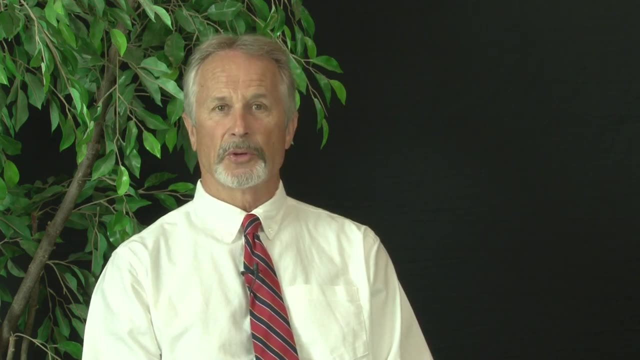 how much will sea level rise over the next century? Although we have global sea level rise values, We know from place to place that those values will vary depending on offshore oceanographic conditions and whether the land is rising or sinking or is tectonically active. 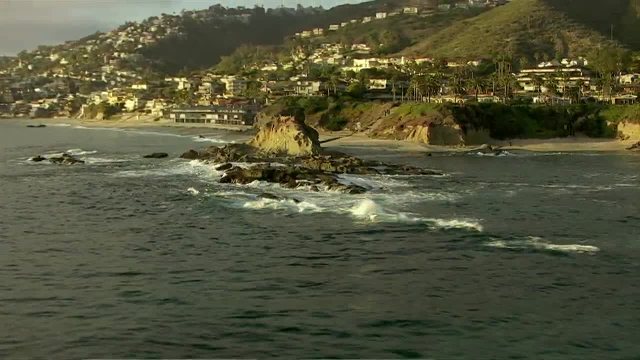 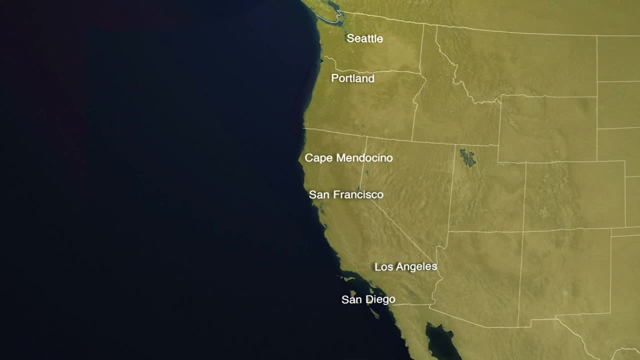 And along the west coast we know we have an active coastline such that the land has been rising and sinking which affects those local sea level rise values. From San Diego north to Cape Mendocino, we know the coast of California which is the 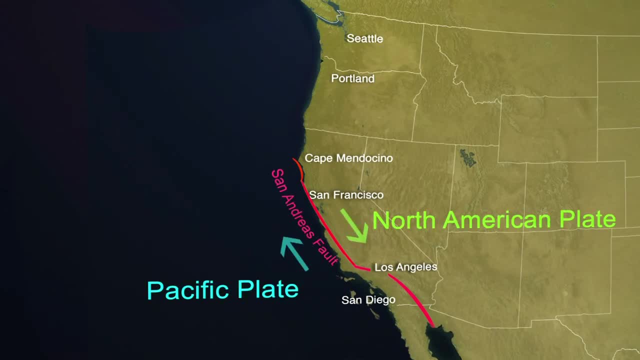 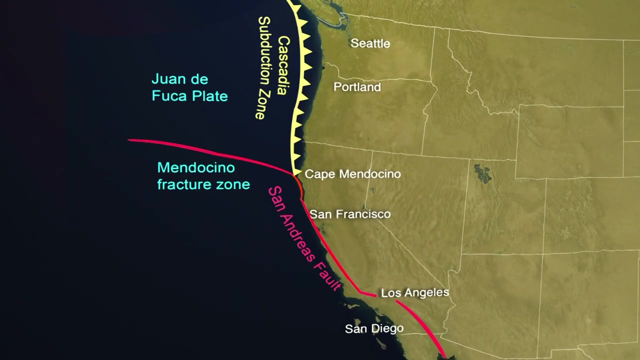 Pacific plate is sliding alongside the San Andreas Fault with very little vertical motion along the coastline, such that sea level from tide gauges over the last century is close to the global number, about four to eight inches North of Cape Mendocino, along the coast of Northern California, Oregon and Washington. 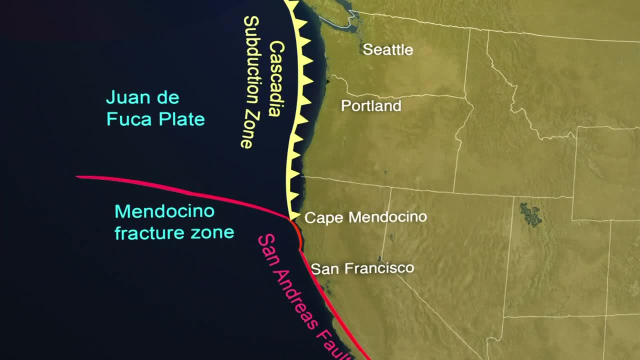 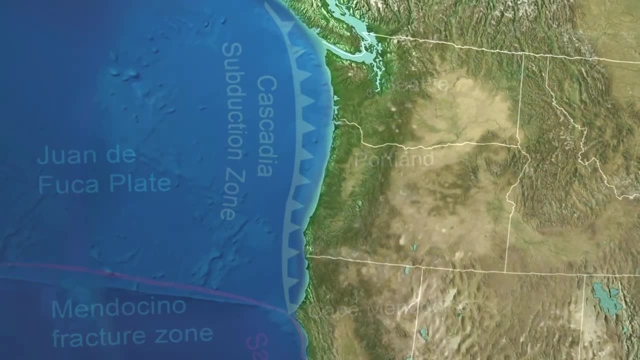 however, the land has been slowly rising, such that many of the tide gauges actually show a small drop in sea level over the last century or so. This region lies along the Casablanca. This is the Cascadia subduction zone where the Juan de Fuca plate descends or is subducted. 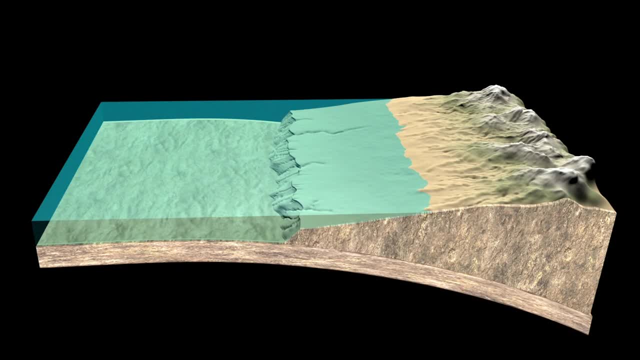 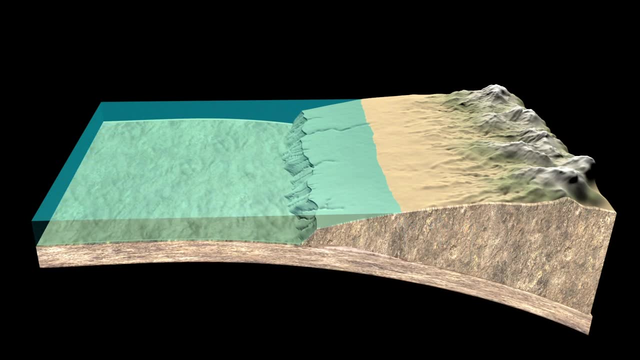 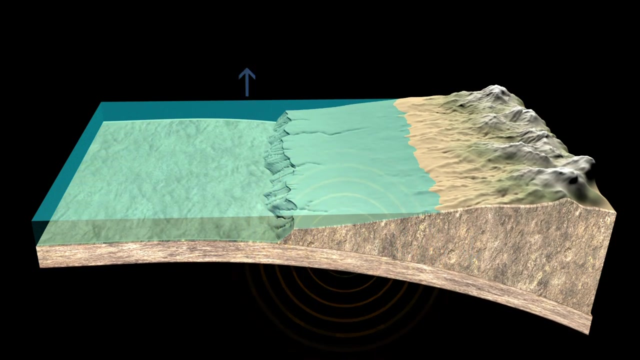 beneath the North American plate. This builds up seismic strain along the coast, which actually pushes the land upward and explains why sea level in the region has dropped, even as global sea level has risen. This could all change very rapidly, however, if we have a large offshore earthquake, which 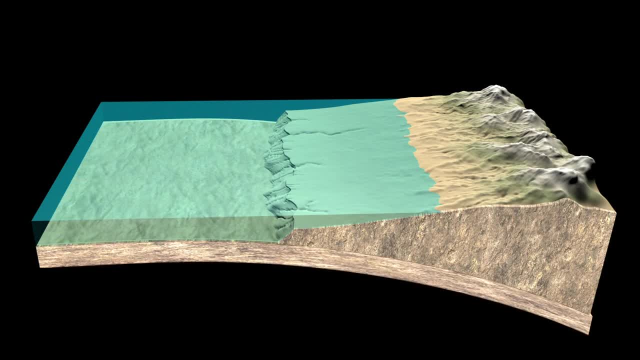 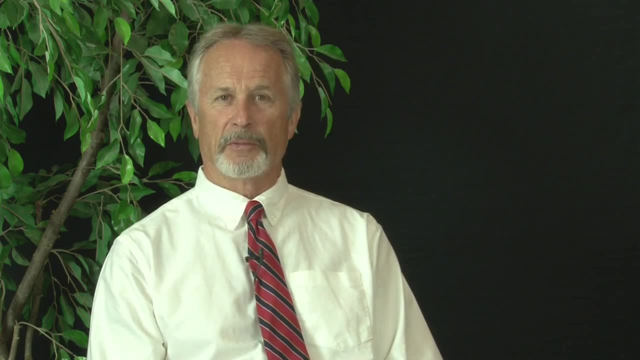 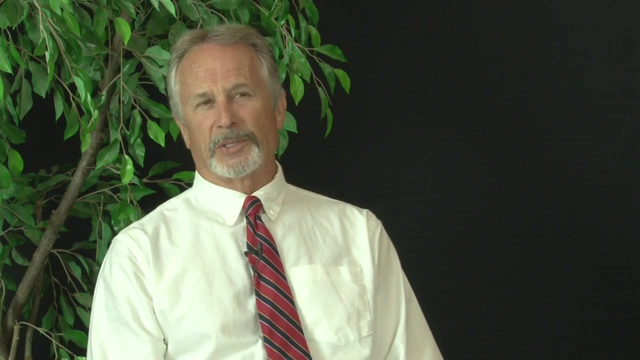 could cause rapid subsidence and therefore an instant rise in sea level. Standards and projections of both climate change and sea level rise indicate that sea level rise is going to continue to rise well into the future. There are uncertainties, however, and that makes precise predictions difficult. 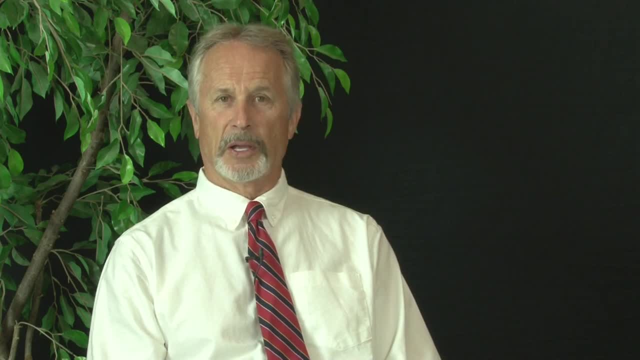 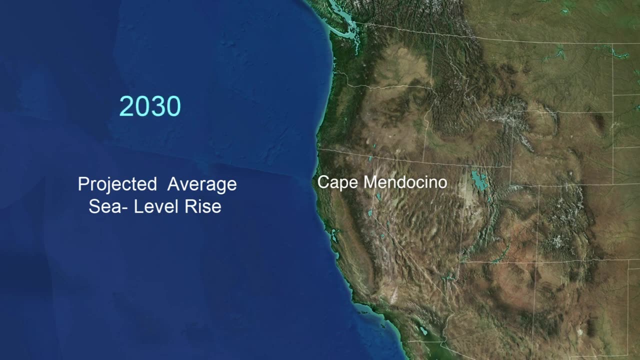 The further we go out in time, the greater those uncertainties become. The committee projected future regional sea levels, and they vary along the West Coast. By 2030, our average sea level rise. values for the area south of Cape Mendocino are projected. 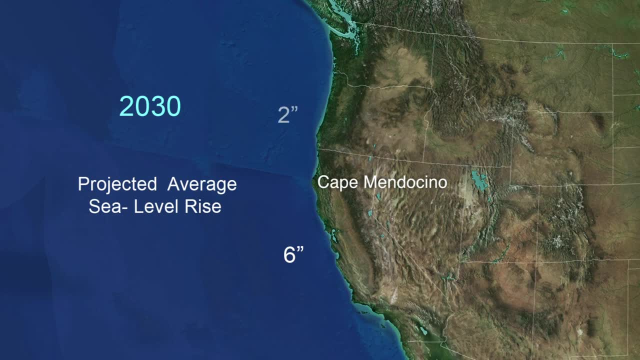 to be about six inches. Well, to the north, only about two inches of rise is expected because the coastline is slowly rising. By 2050, we project 12 inches of rise to the south and six inches to the north along the Oregon and Washington coasts. 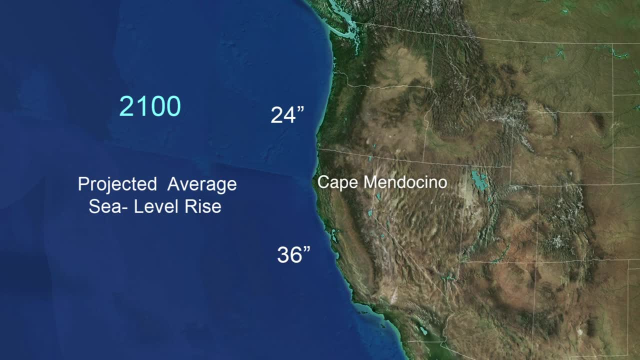 And by 2100,. average values of 36 inches are projected along the California coast and 24 inches north of Cape Mendocino. These are average values, however, and the actual values could be significantly higher or lower For some perspective. 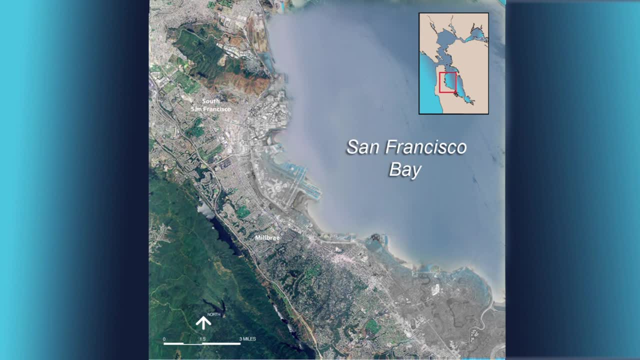 Let's look at an example of a few examples of the current sea levels. The two major international airports in San Francisco Bay, San Francisco and Oakland were built on fill only a few feet above sea levels, such that 16 inches of sea level rise, which 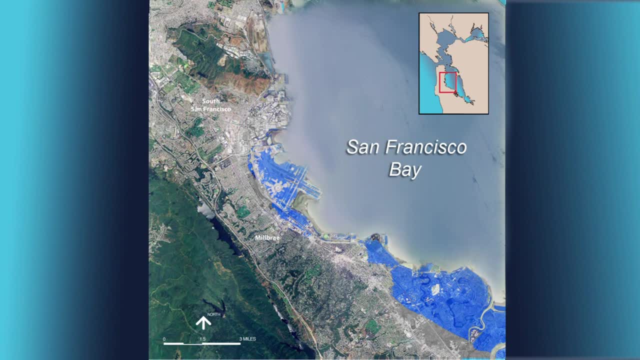 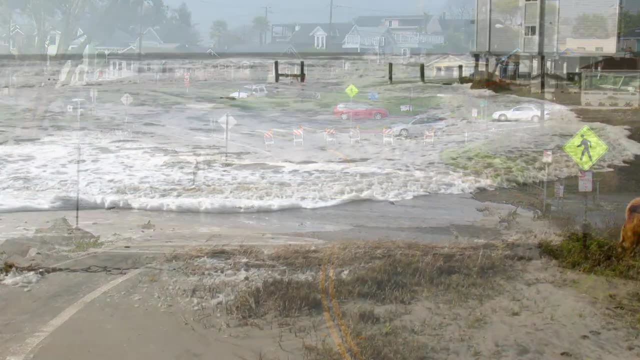 could happen in the next several decades would begin to inundate those runways. Many west coast communities already experience coastal erosion, flooding and inundation, and loss of wetlands due to El Nino-elevated sea levels, the impacts of large waves at times. 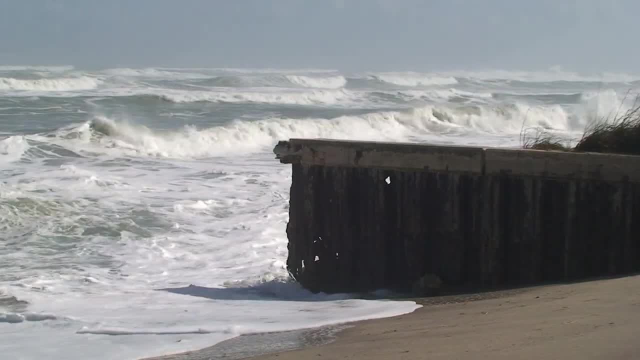 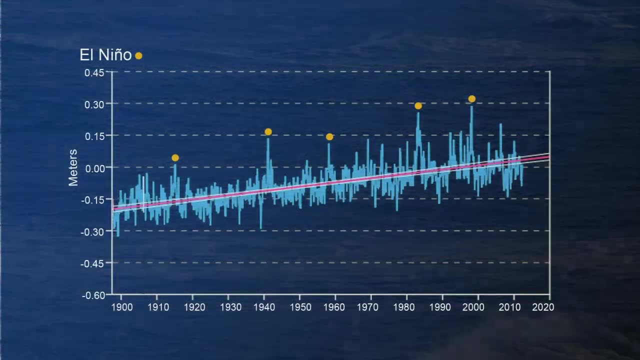 of high tides and a slowly rising sea level rise, But the reality is that there is still a lot of real damage to be done to these major sea level. The water levels reached during these short-term events have exceeded mean sea levels projected for 2100.. Thus, at least for the next several. 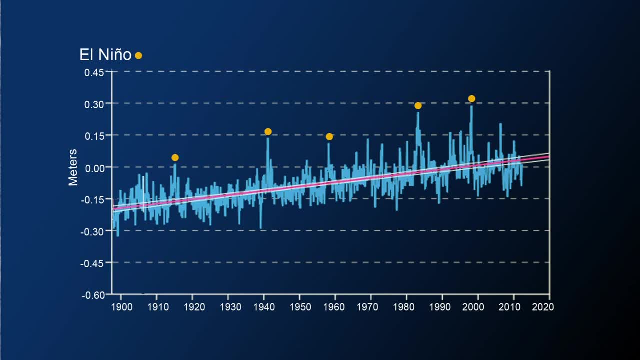 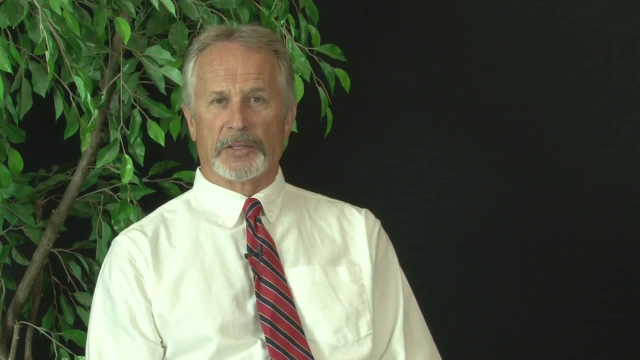 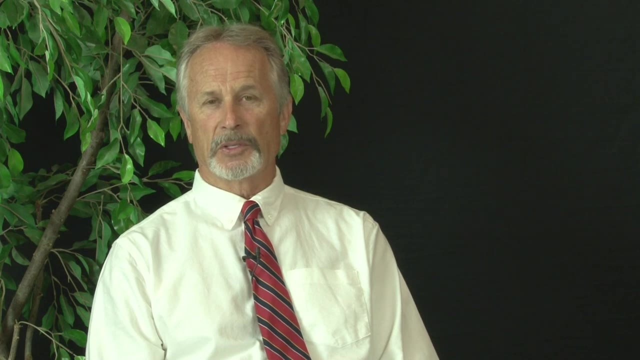 decades. these events are a greater hazard for the West Coast than the climate-driven rise in sea level. It's very likely that in the future, as sea level continues to rise, that the impacts of those events will get greater in magnitude, and also likely they will increase in frequency as we move into. 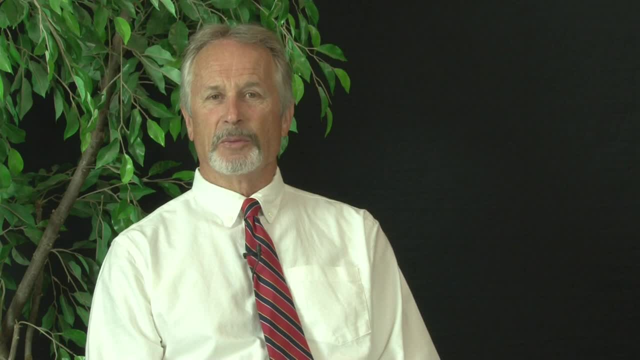 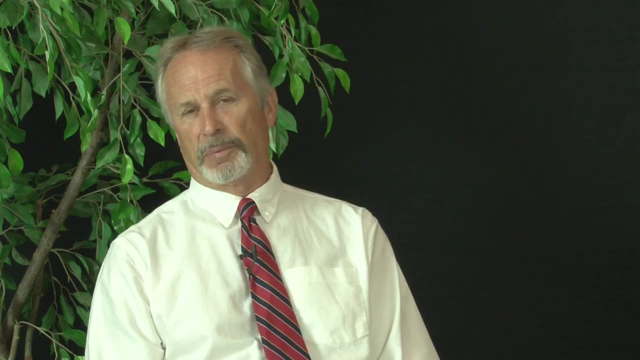 the future. Coastal communities need to begin to understand these processes and what these sea level rise indicate to them, and plan accordingly.